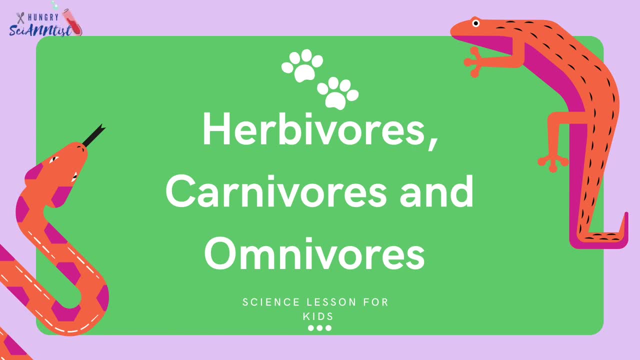 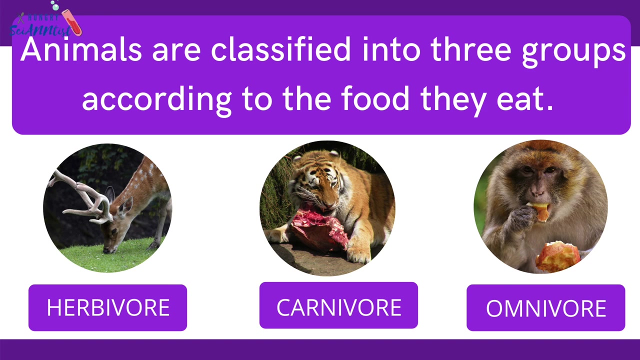 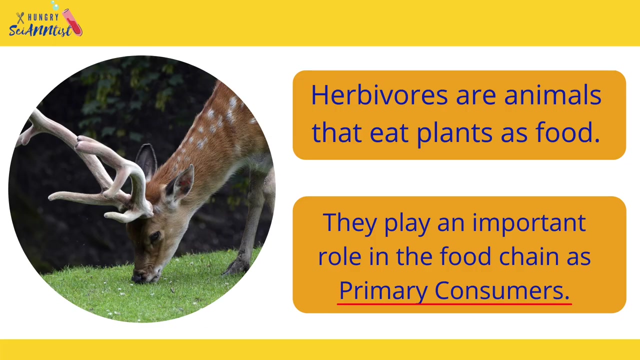 In this video, we will learn about herbivores, carnivores and omnivores. Animals are classified into three groups. according to the food they eat, They are grouped into herbivore, carnivore, omnivore. Herbivores are animals that eat plants as food. 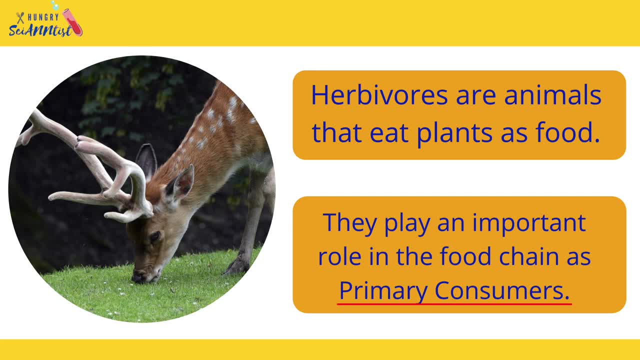 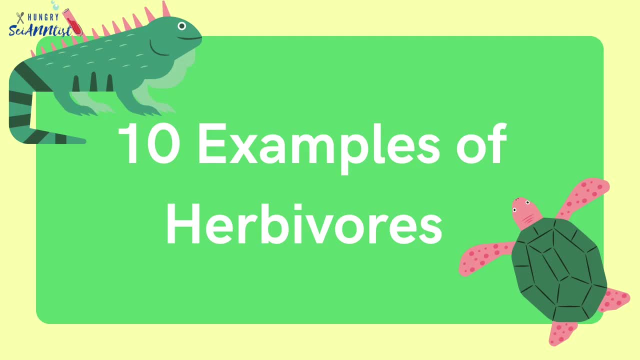 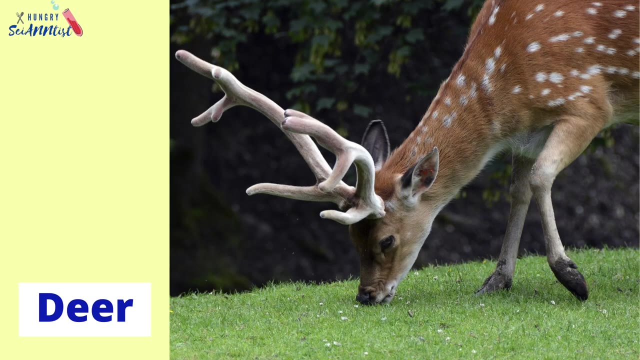 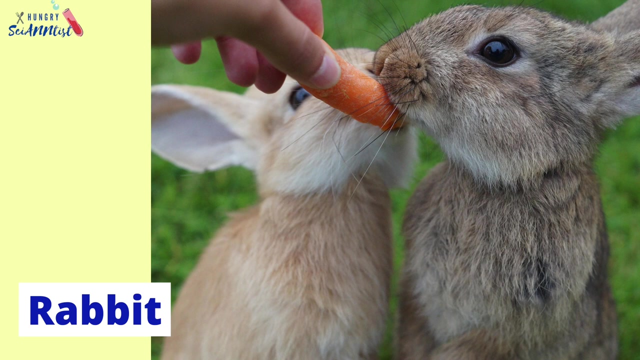 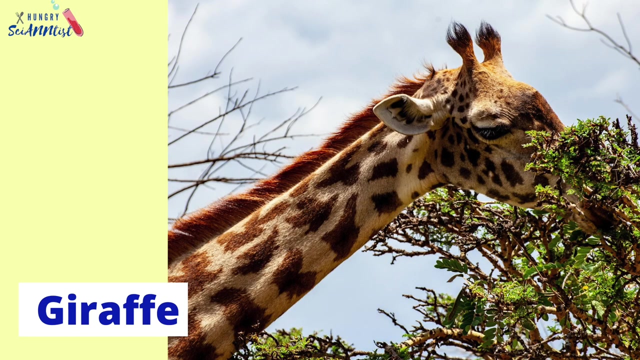 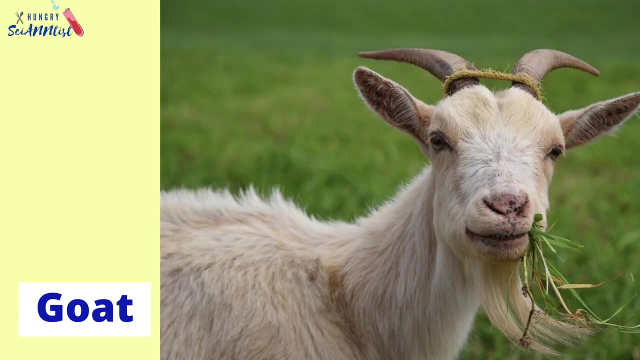 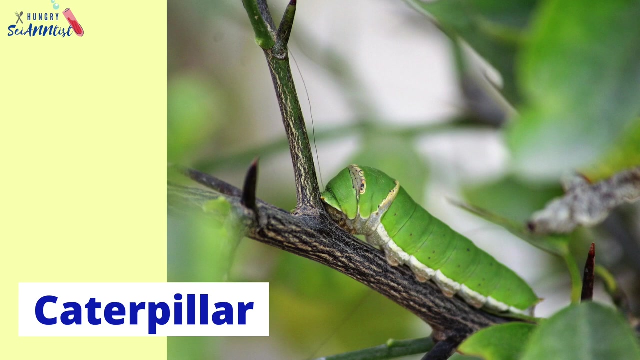 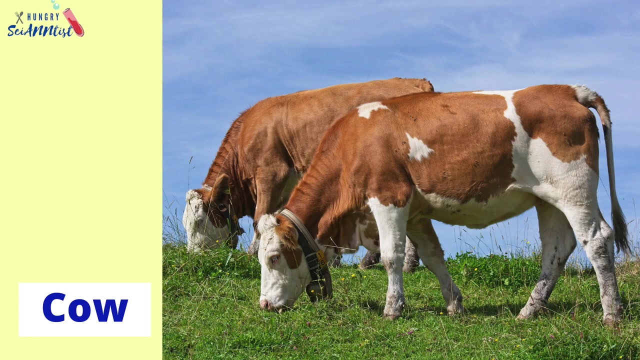 They play an important role in the food chain as primary consumers. Examples of herbivores: Herbivores are plants that eat food that can killslice than humans. Herbivores are animals that eat plant-based home-grown food. Herbivore are animals that belong to a community of €10 a month. 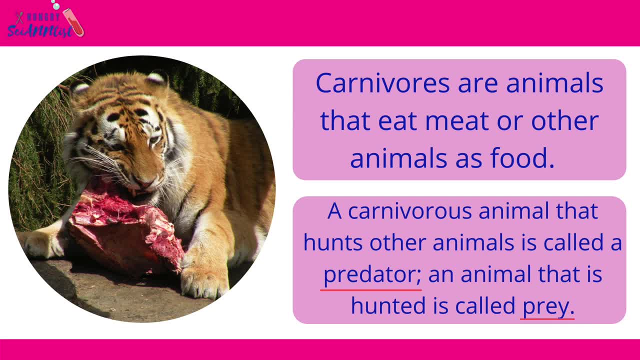 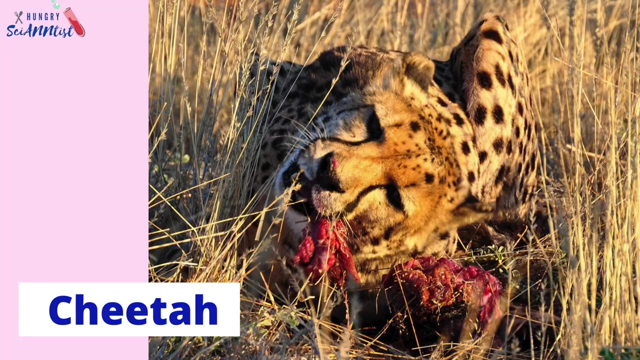 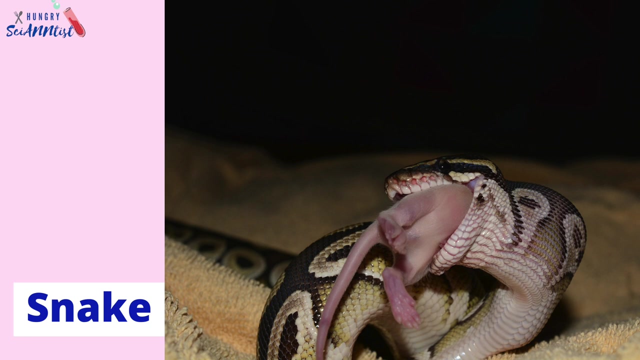 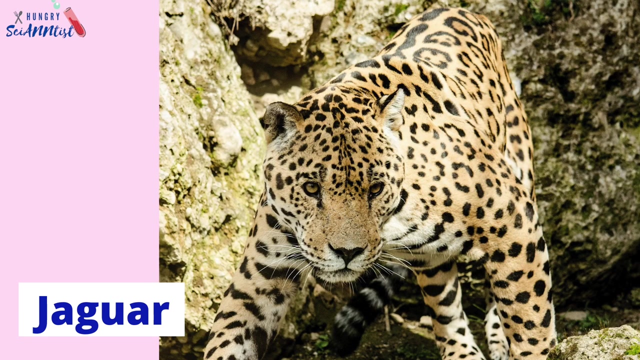 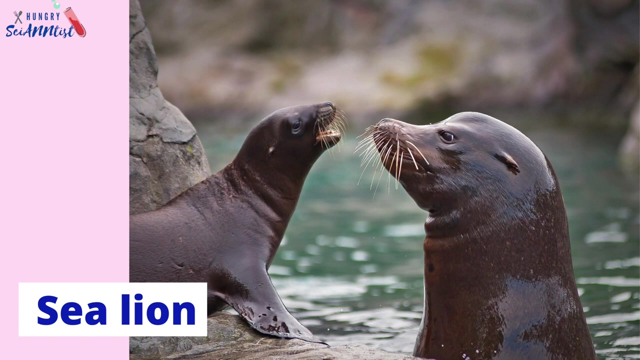 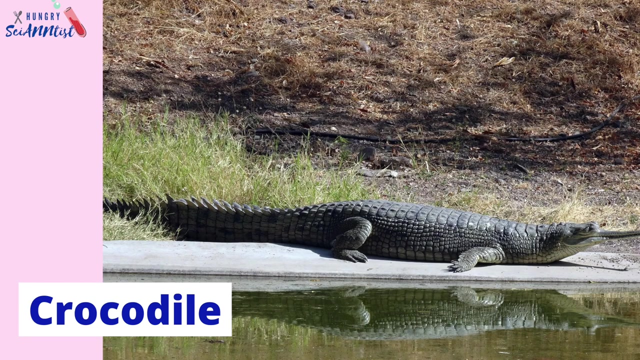 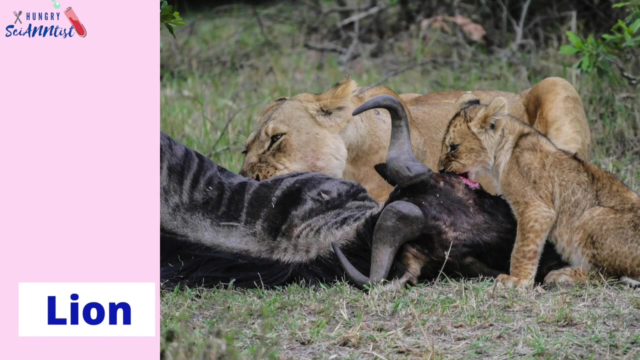 same as moyens for consumption. Carnivores are animals that eat meat or other animals as food. A carnivorous animal that hunts other animals is called a predator. An animal that is hunted is called prey. Examples of carnivores. A carnivorous animal that hunts other animals is called a predator. 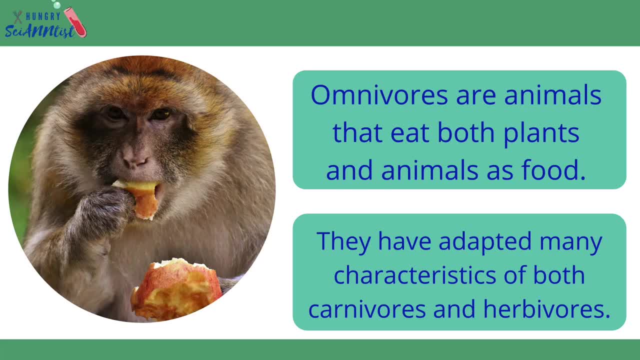 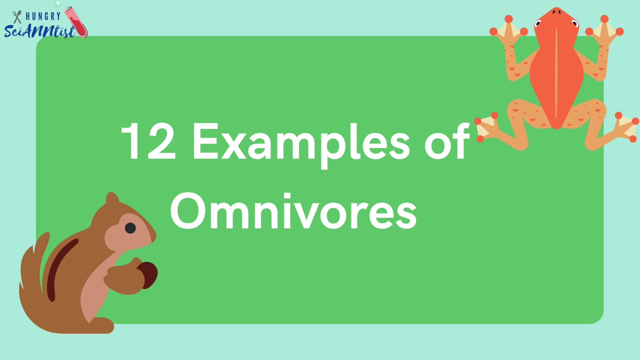 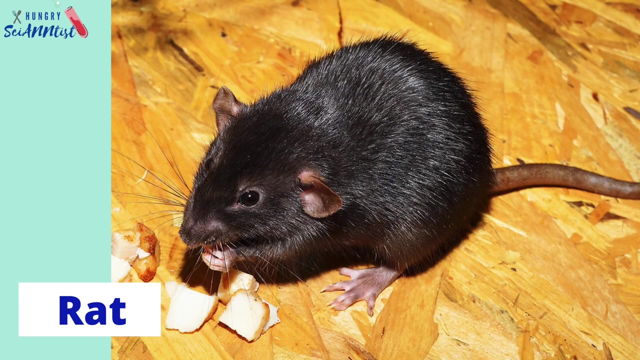 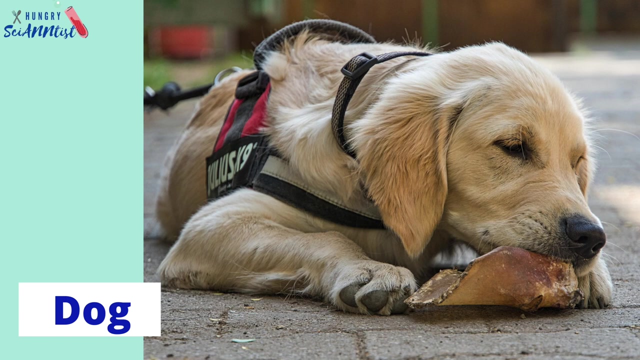 Omnivores are animals that eat both plants and animals as food. They have adopted many characteristics of both carnivores and herbivores. Examples of omnivores. This is an example of omnivores that hunt for food. An omnivore that is hungry until morning.